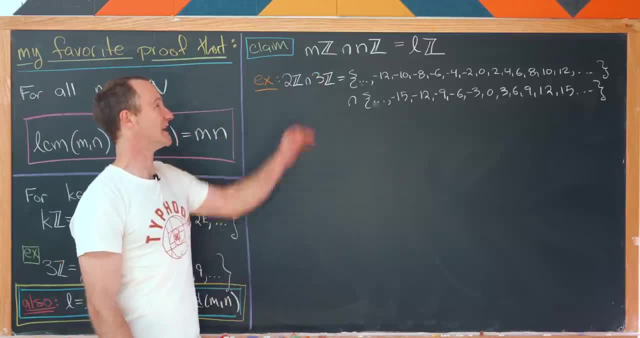 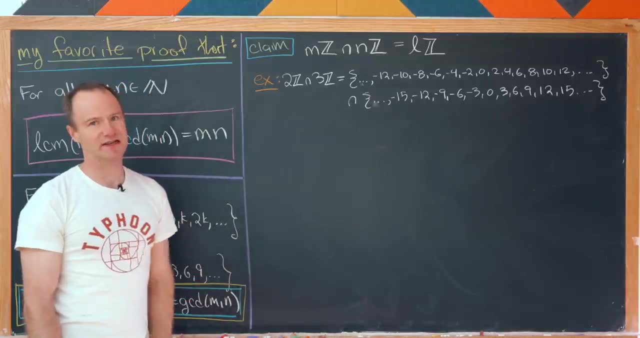 And now our first claim will be to prove that if we intersect MZ with NZ, we get LZ. So let's look at a little example of that happening, just so that we have a feel for what's going on. Let's take 2Z intersected with 3Z, But let's recall that 2Z is all multiples of. 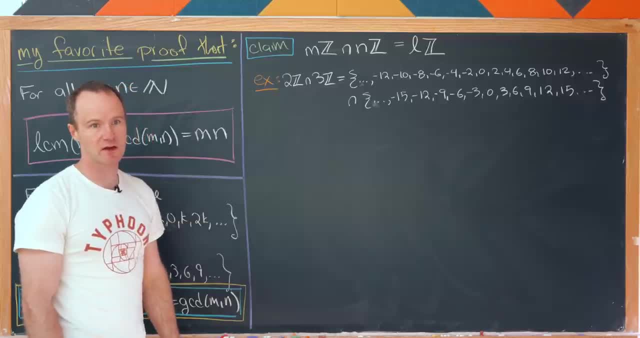 2,, whereas 3Z will be all multiples of 3.. So really, you think to yourself: well, what's a multiple of 2 and a multiple of 3?? Well, it has to be a multiple of 6.. But let's do the intersection. 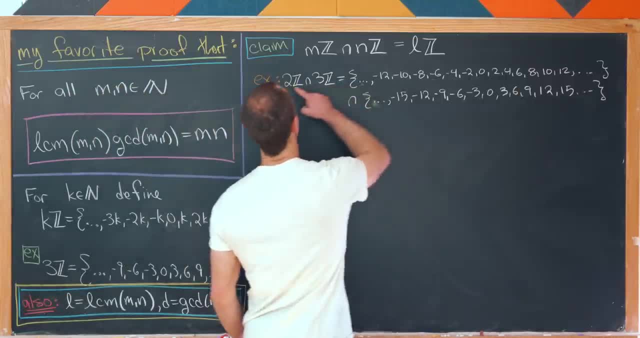 just to be sure. So again, if we intersect MZ with NZ, we get LZ. So let's look at a little example, going through all of the multiples of 2 and all of the multiples of 3.. Let's maybe underline the. 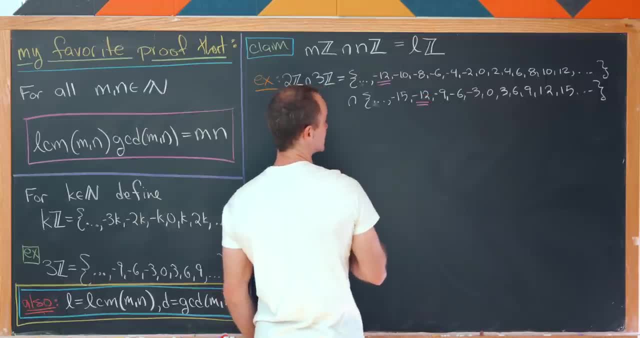 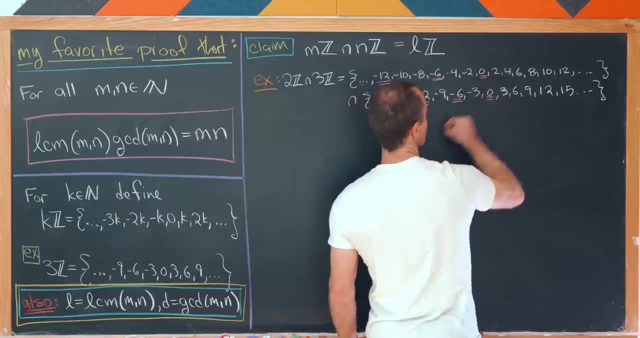 numbers that show up in both sets. So we've got minus 12.. That's in both of these sets. Minus 6 is in both of these sets. 0 is in both of these sets. 6 and 12 are in both of those sets. 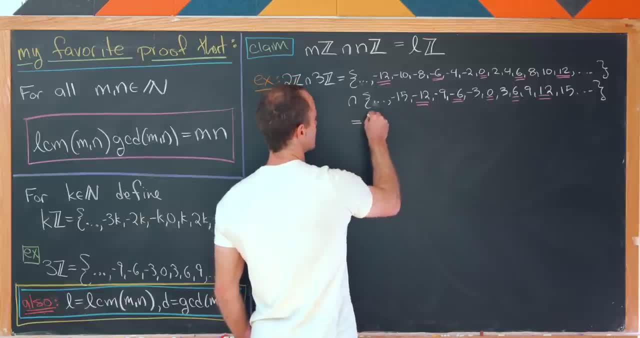 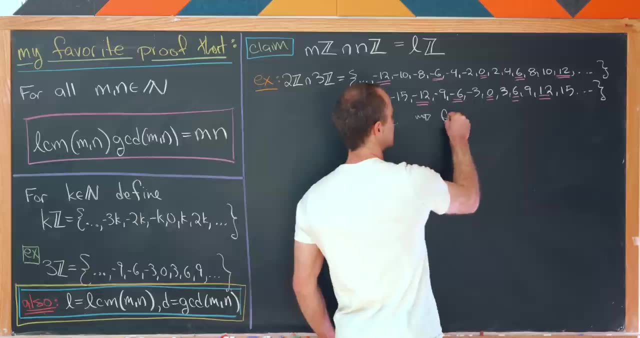 So it, you know, seems like all of the multiples of 6 will be in both of those sets. So let's look at a little example of that. So, let's look at a little example of that. But this makes sense in this case because 6 is most definitely equal to the LCM of 2 and 3.. 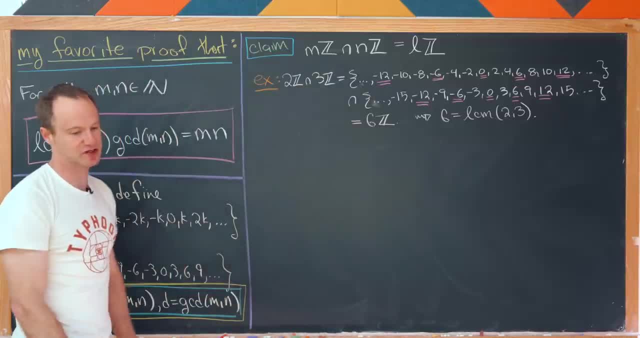 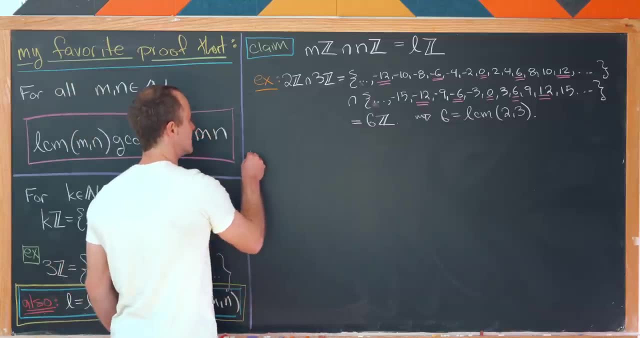 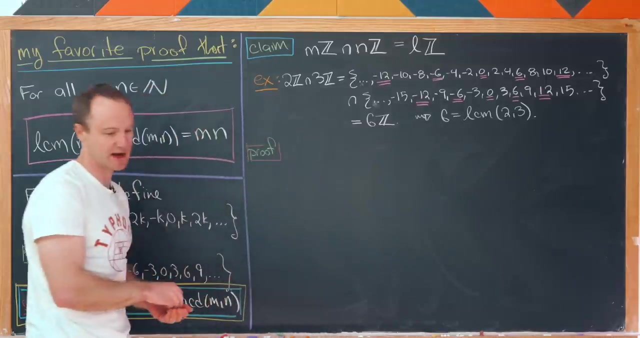 2 and 3 are so-called relatively prime, so their LCM is just their product. So let's maybe sketch a little bit of a proof of what's going on here. And I say a sketch because perhaps really we'll only do, you know, one side of the inclusion. I'll leave maybe the other side as a homework exercise. 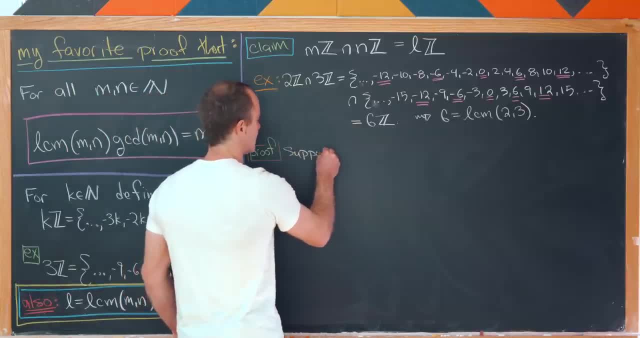 So let's look at a little example of that. So let's look at a little example of that. So let's look at a little example of that. So let's maybe suppose that we have A is inside MZ, intersected with NZ, But then what that means. 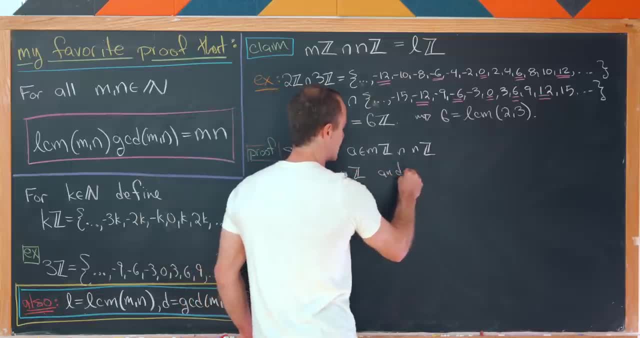 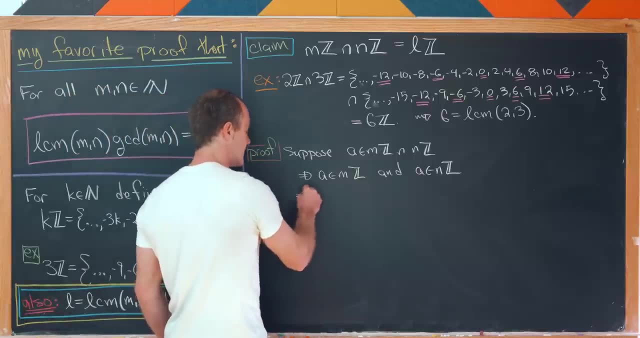 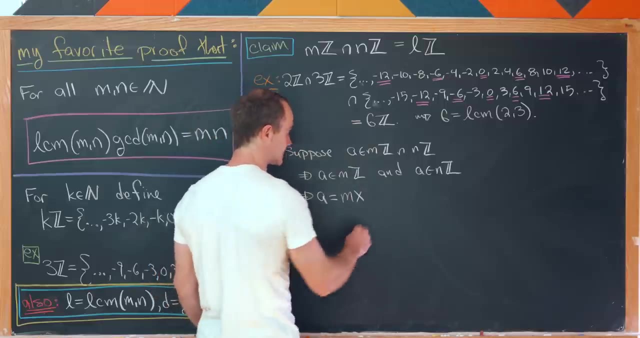 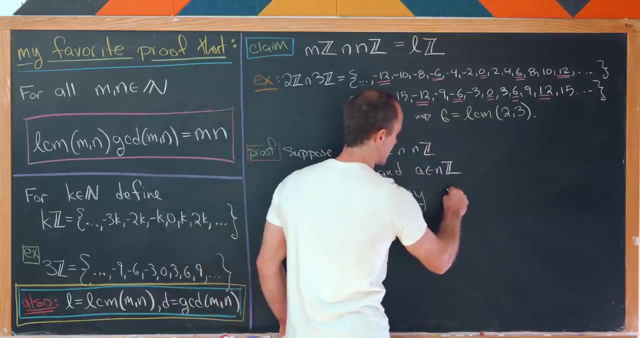 is that A is in this set MZ and A is in this set NZ. You know, that's the definition of intersection. But then we see that A must be a multiple of M, So that means A equals MX And A must be a multiple of N. That means A must be equal to N times Y, And this is where X and Y 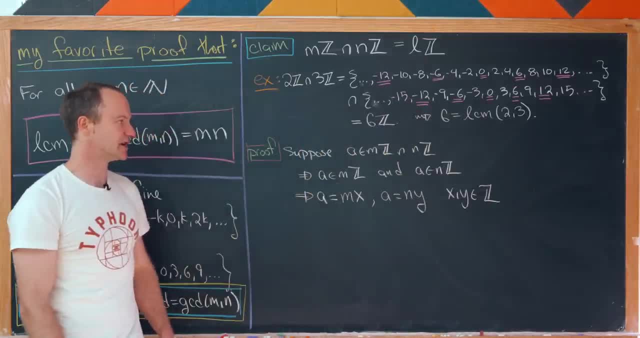 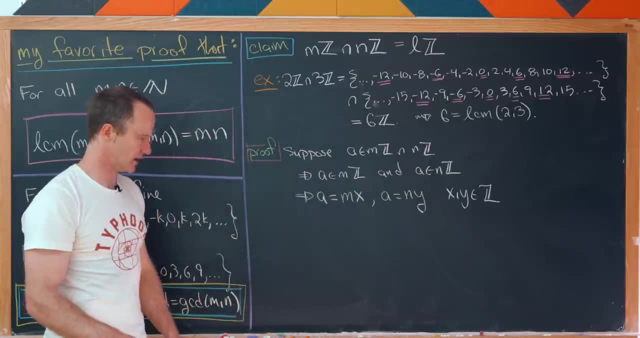 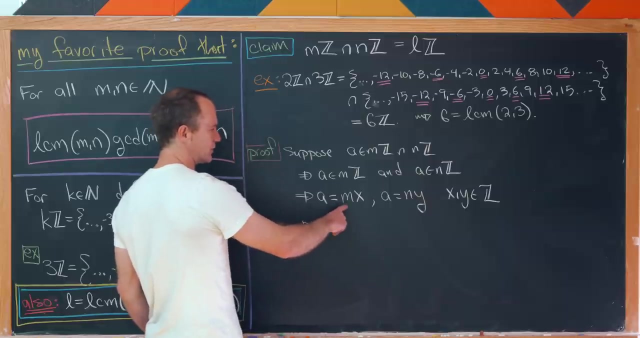 are integers. Again, how do you get inside the set MZ? Well, you're a multiple of M. How do you get inside the set NZ? Well, you are a multiple of N. Okay, but now let's look at this. This means that A is a multiple of M and a multiple of N. 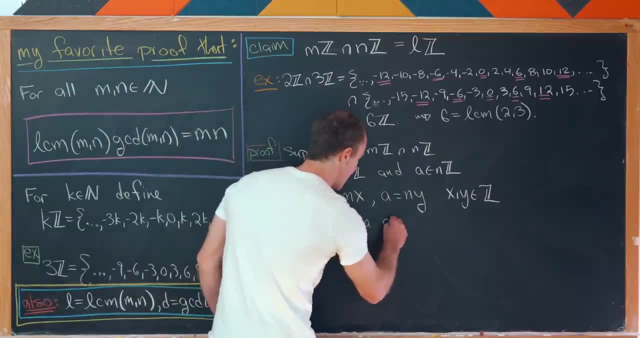 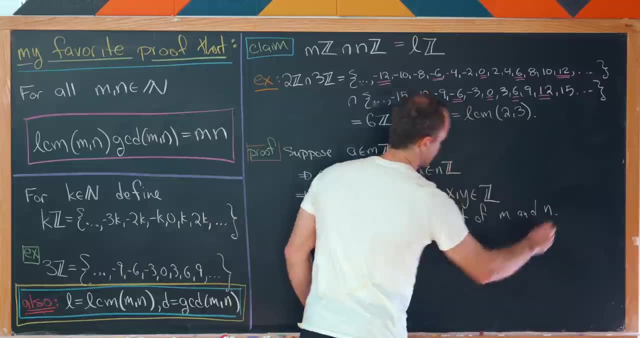 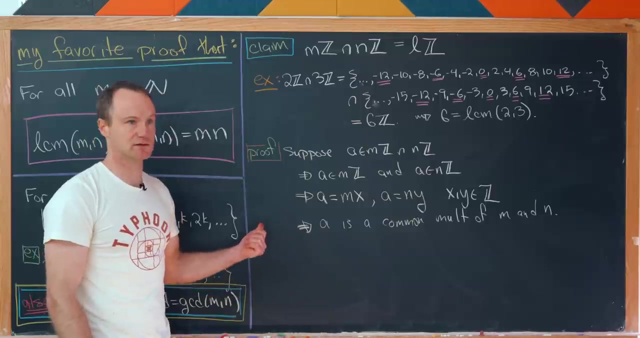 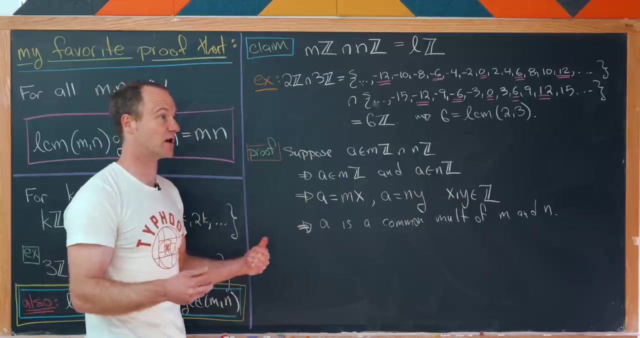 But that means that A is a common multiple of M and N. What's maybe the defining property of the least common multiple? Well, it's the least common multiple, But how do we measure that leasedness or that smallness when we're talking about divisibility, which we're really talking? 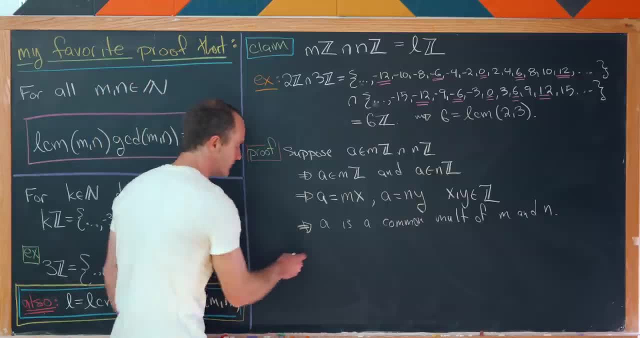 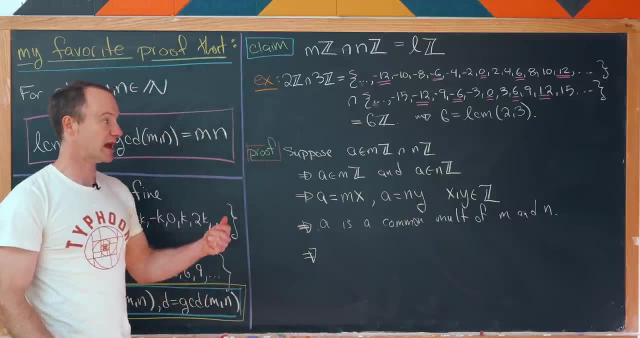 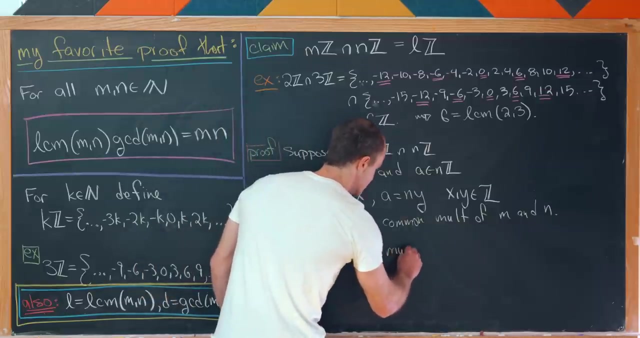 about here, And we measure it By saying that if you have a common multiple of M and N, then it must be a multiple of the least common multiple of M and N. So let's write that here. So A is a multiple of the LCM of M and N. 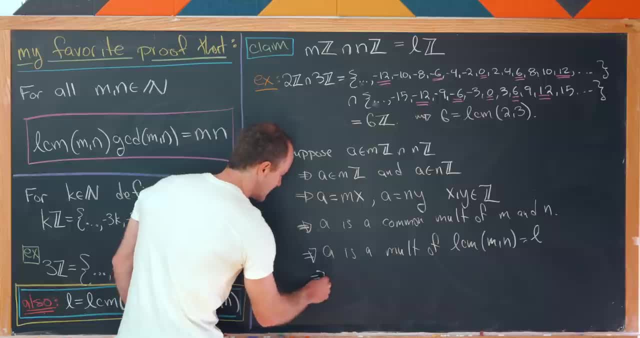 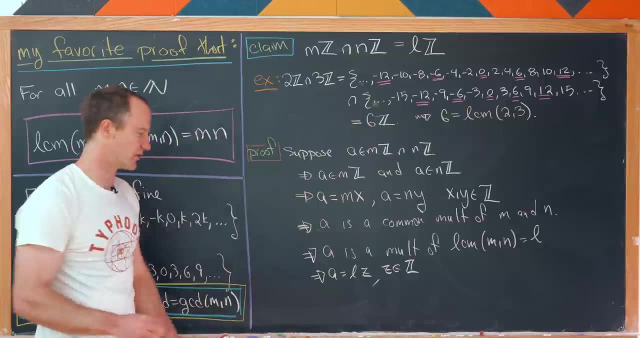 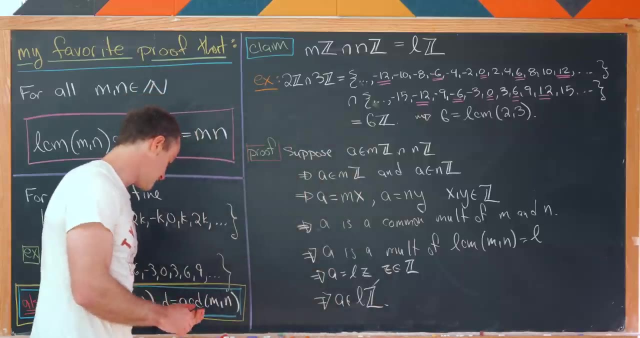 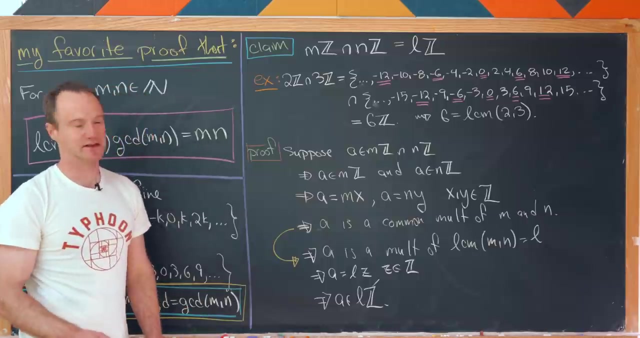 which we called L, But that means that A equals LZ for some integer Z. That's the definition of it here, But that means that A is, in this set, LZ. Now, you might be a little spooked out at this right here, but this is in fact just the definition of the LCM, If you're a common. 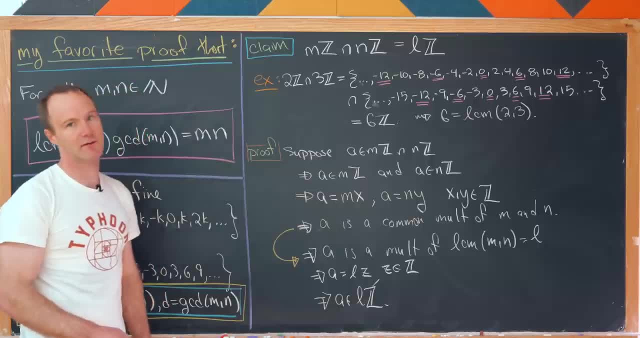 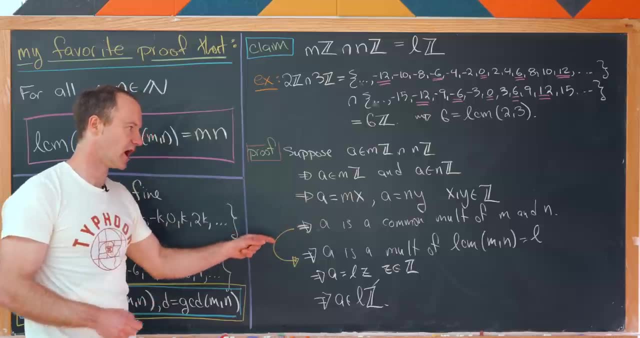 multiple of two numbers, then you must be a multiple of the least common multiple of those two numbers. And in fact, maybe under the hood, what's happening is, if a common multiple is not a multiple of the LCM, then you can produce. 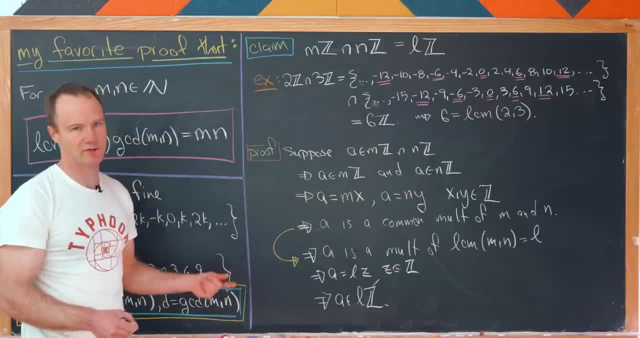 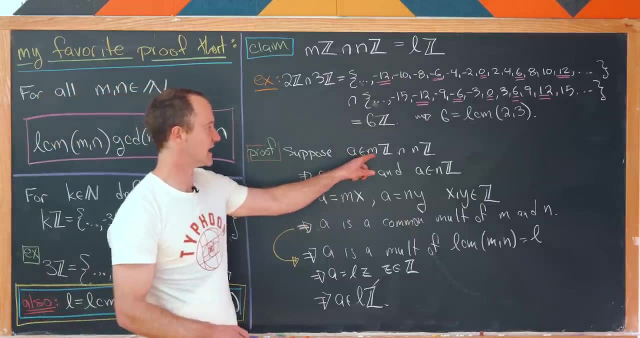 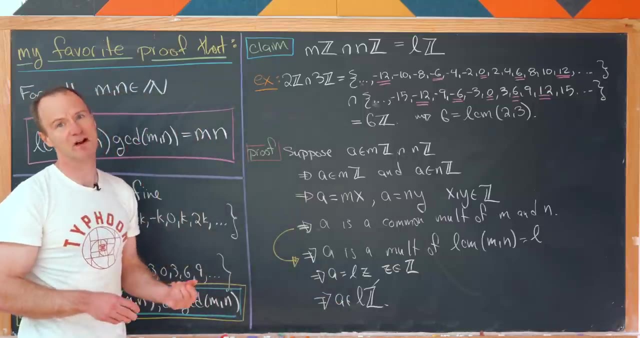 something smaller than the LCM. That's in fact a common multiple, which would contradict the LCM-ness of that. Okay, so anyway, that's one direction here That shows that MZ intersect NZ is a subset of LZ. I'll maybe leave the other direction for you. It's fairly straightforward. 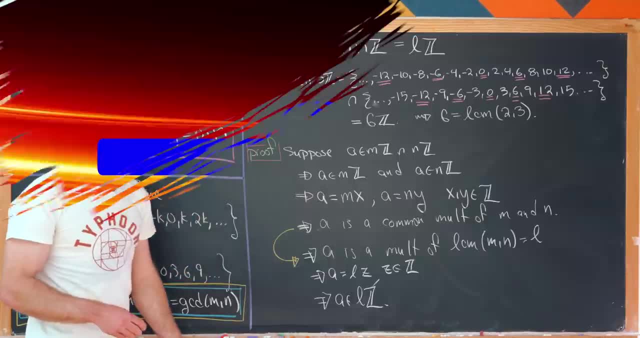 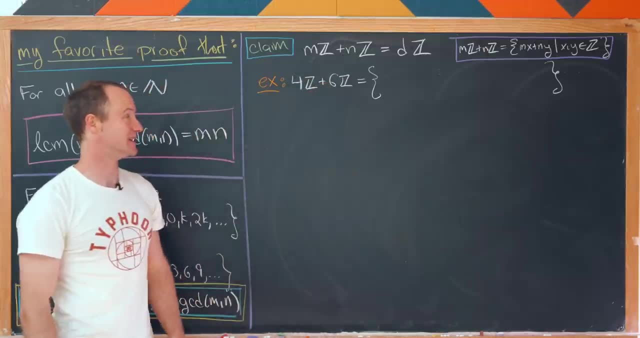 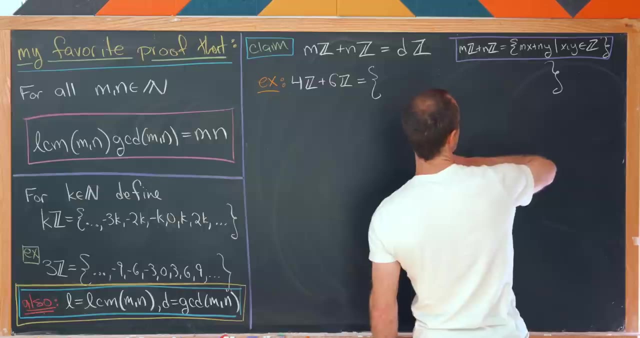 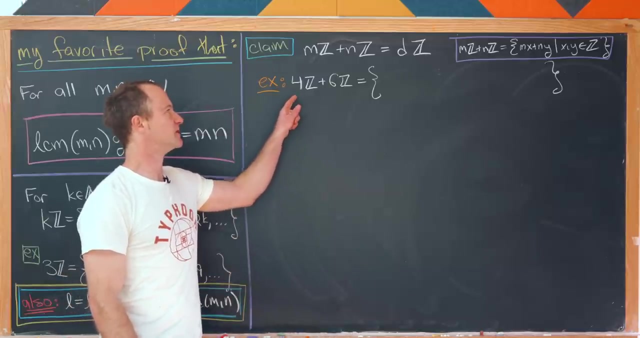 And now let's move on to another similar statement, So the next object which will be a piece of our set. So by that I mean the set containing everything of the form MX plus NY, where X and Y are both integers. So let's build a little bit of an example here. So we'll look at 4Z plus 6Z And then 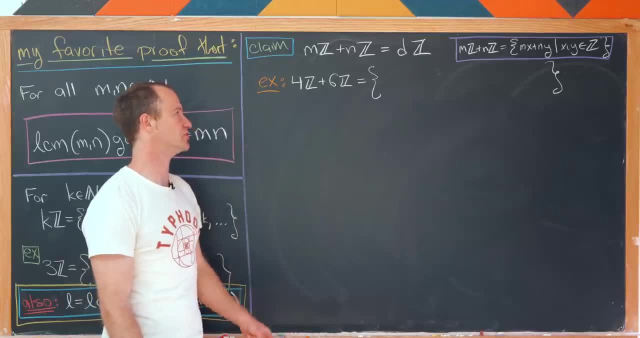 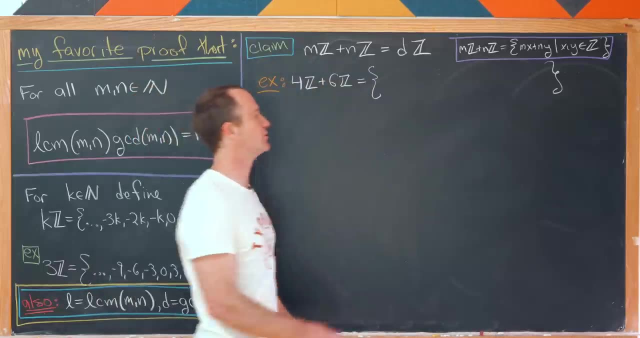 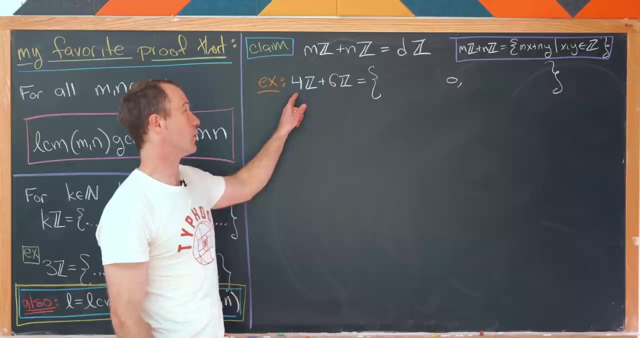 we'll just like semi-randomly pick some integers to choose for X and Y and then get some elements of this set. So notice, we can choose X and Y to both be zero and that'll tell us that the set is zero is inside this set. Furthermore, we could look at like four times negative, one plus six. 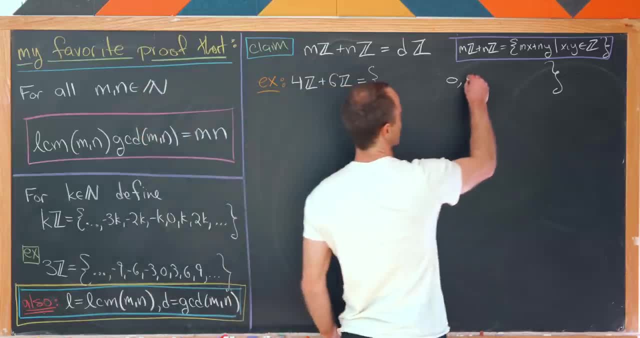 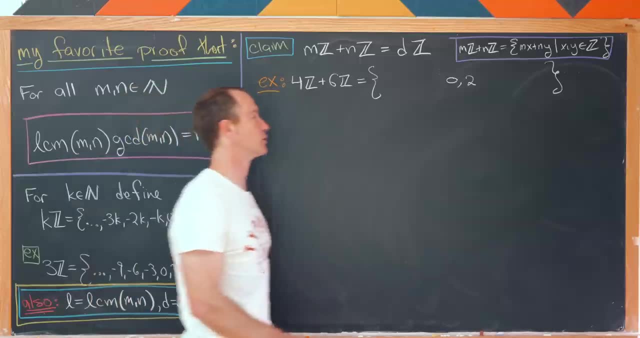 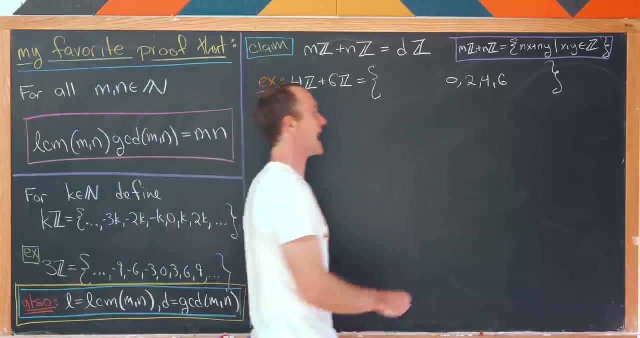 times one, and that'll give us two inside of this set. Or we could in fact take six times zero plus four times one, and we'll get four in this set. And likewise we could get six in this set as well, And it's pretty easy to see that eight is also in this set. So, whoa, it looks like. 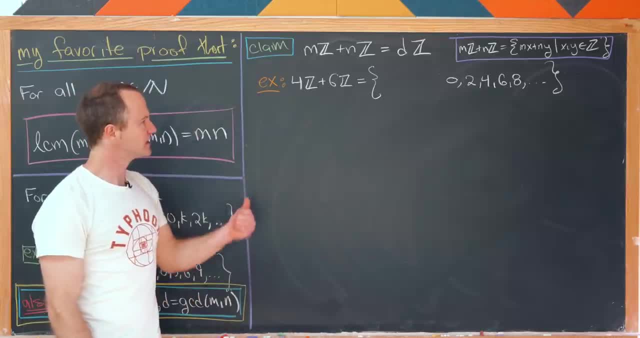 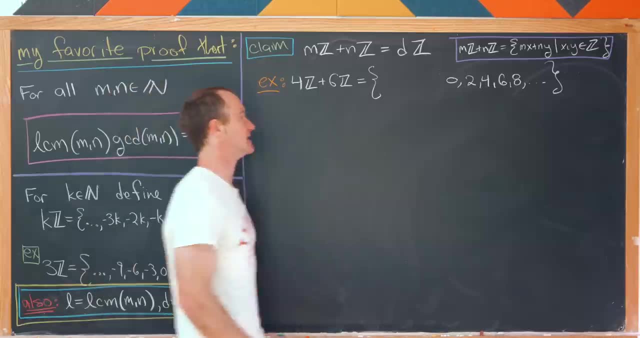 all of the even numbers are in this set. Well, let's go backwards. Can we get negative two in this set? And we can, and that's if we'd attach four to a positive one and six to a negative one. So that gives us negative two in this set. Negative four can get in this set by attaching. 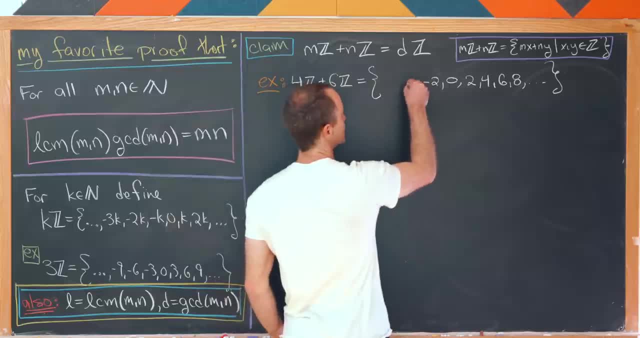 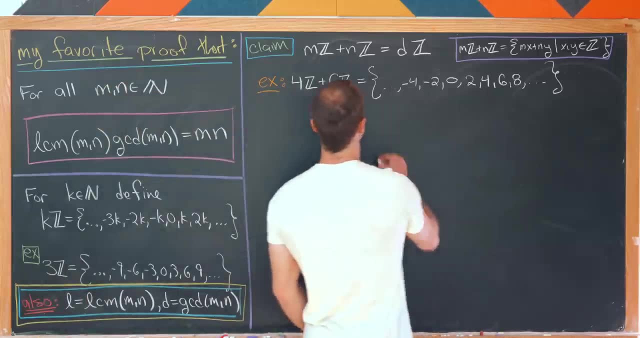 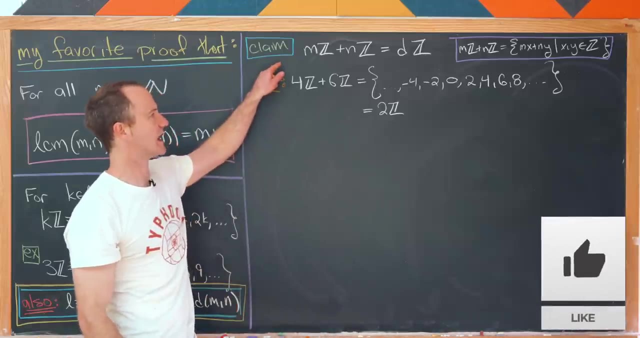 four to a negative one and six to a zero. So then we've got negative four and then back that way. Now it really looks like it's all even integers. but all even integers can be written as two times z. But now let's go up to our claim here, which is the structure of this. 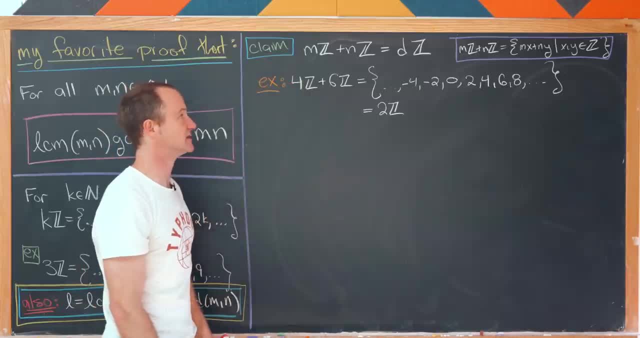 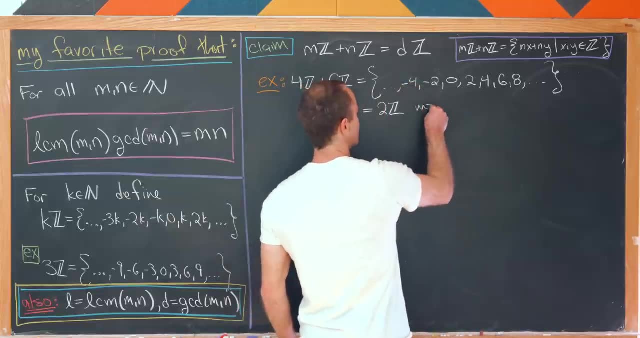 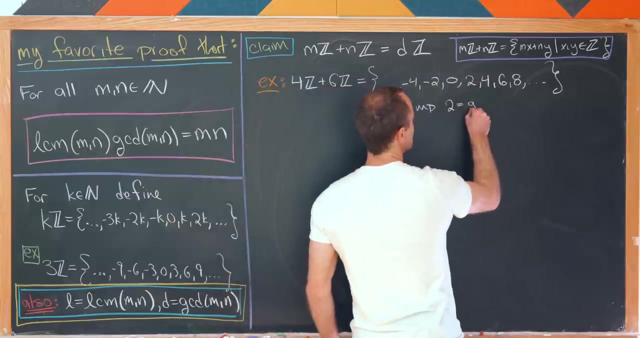 type of set. It says that m times z plus nz is equal to dz, where let's recall that d was the gcd. Well, does this work with this? you know example that we've been working with. And it does, because notice that two is in fact the gcd of four. with six It is the two with six. So that's the gcd of four with six, And that's the gcd of four with six. So that's the gcd of four with six, And that's the gcd of four with six, And that's the gcd of four with six. 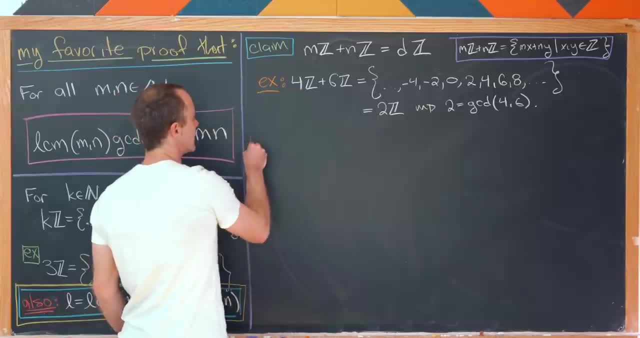 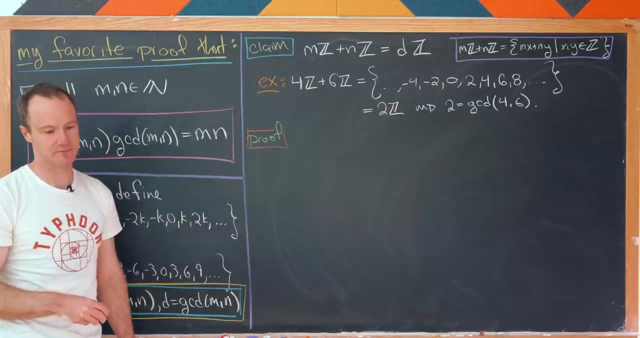 greatest common divisor. So now let's do another little sketch of this proof And then we'll essentially have all of the pieces that we need. Well, we're going to use like a mystery big result to really like take it home, But we'll go over that when we get to it. Okay, so let's. 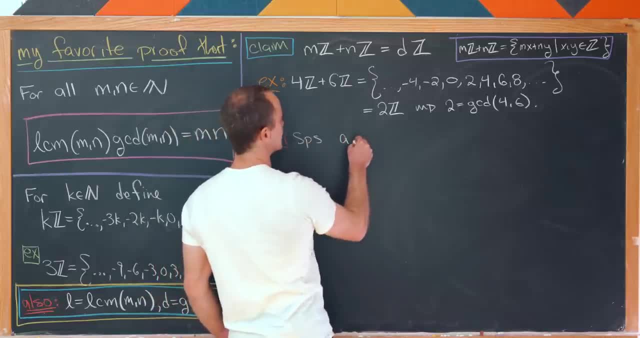 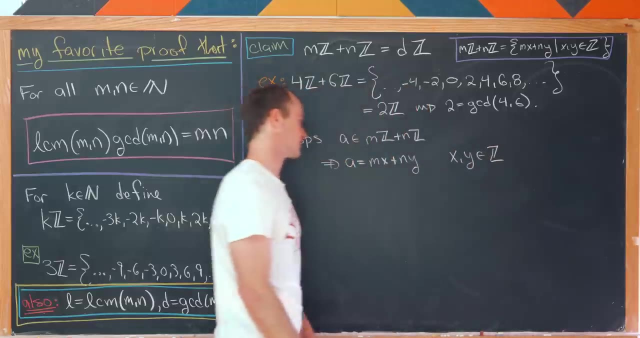 maybe suppose that a is inside of mz plus nz. But what does that mean? That means that a is of the form mx plus ny, where x and y are in the integers. But now, since d is the gcd of m and n, 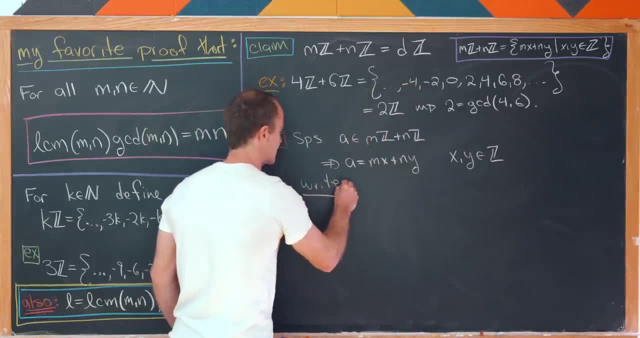 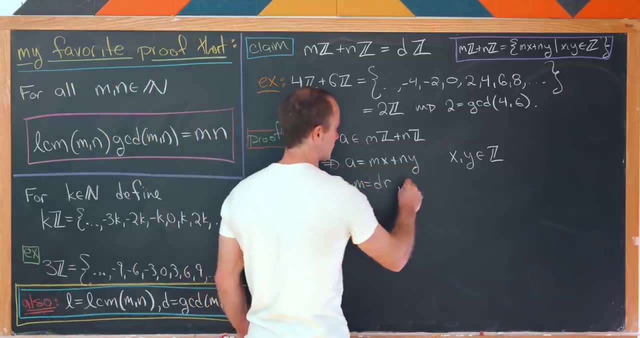 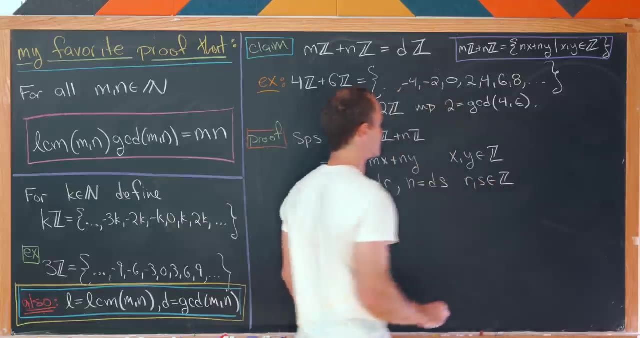 we can write m and n as multiples of d. So let's maybe write m as d times r and we'll write n as d times s And again we'll take r and s to be integers. And, like I said, that's possible because d is a common divisor of m and n. But now, 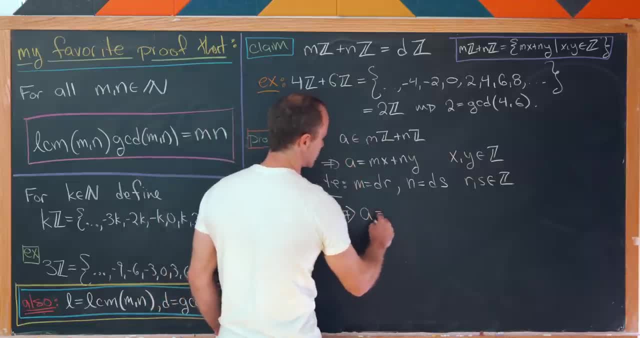 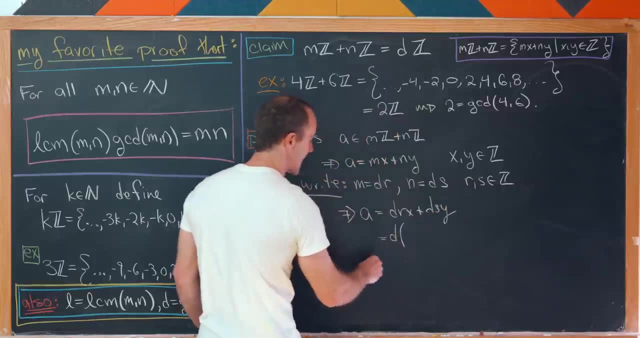 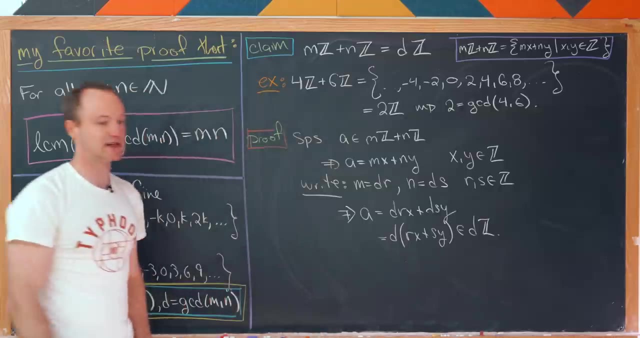 injecting that into this equation, we have a is equal to, let's see, drx plus dsy. We can factor a d out and we'll have rx plus sy, But that's most definitely an element of dz. Okay, so now. 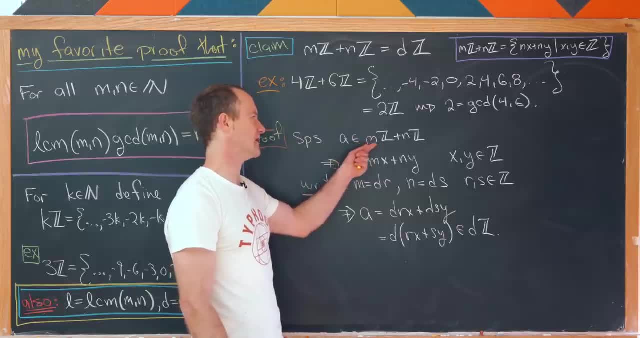 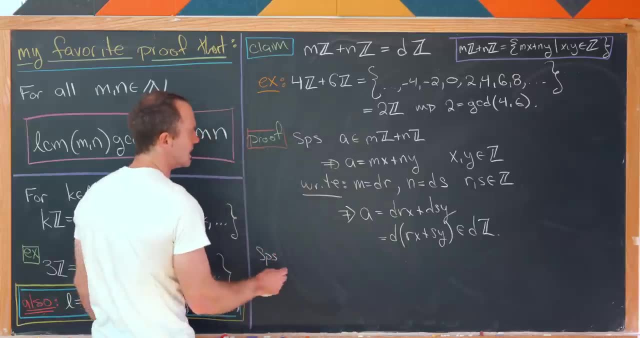 that shows us that we have a common divisor of m and n, And now we're going to be able to write a subset relationship between mx plus ny and dz. Now, how would we go in the other direction? Well, let's go in the other direction, maybe just a bit. We will use a result, but it's 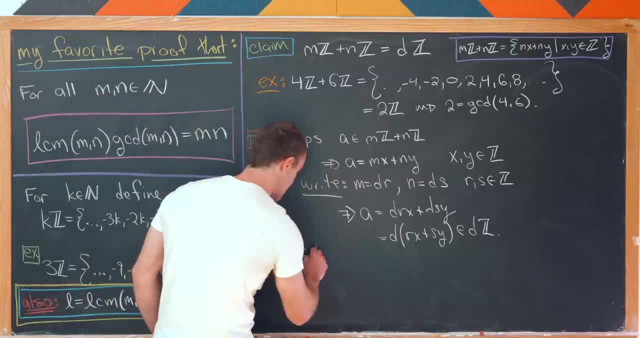 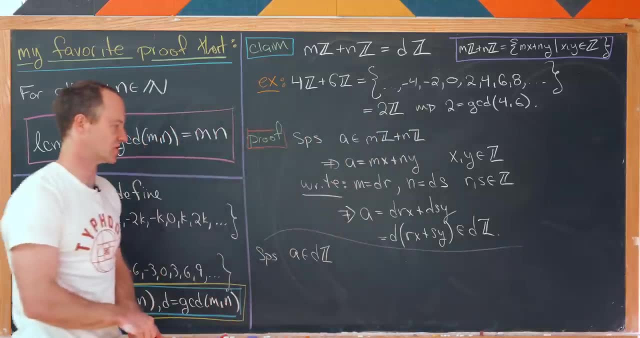 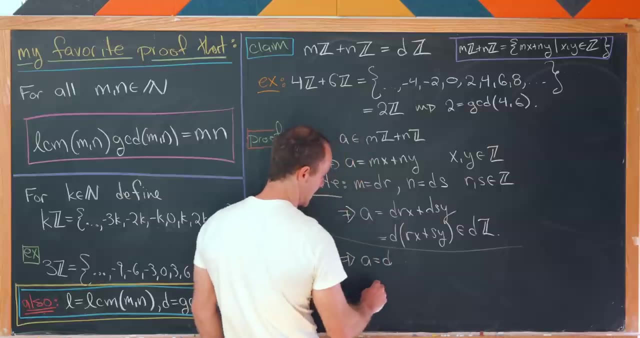 a result. we use on the channel a lot. So let's suppose that a is inside of our set dx, So I'm going to maybe put a line here just to say that we're partitioning this, Okay, so what does that mean? That means that a is equal to d times. 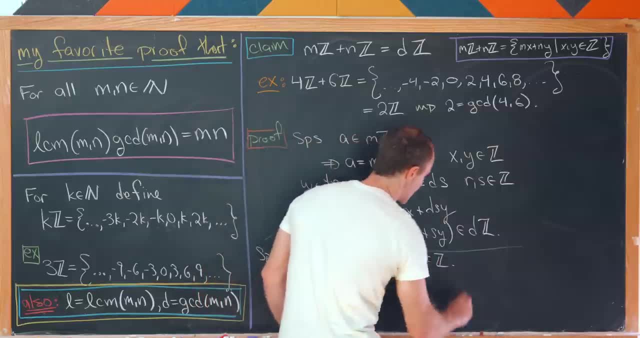 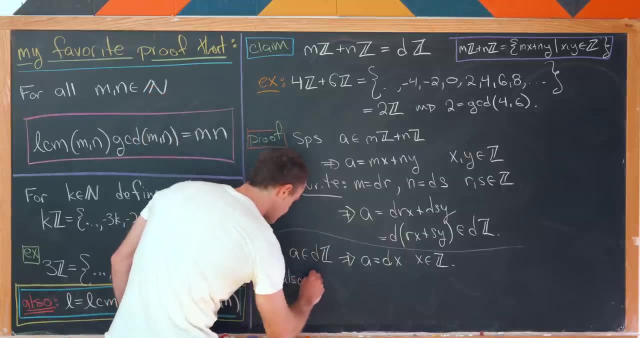 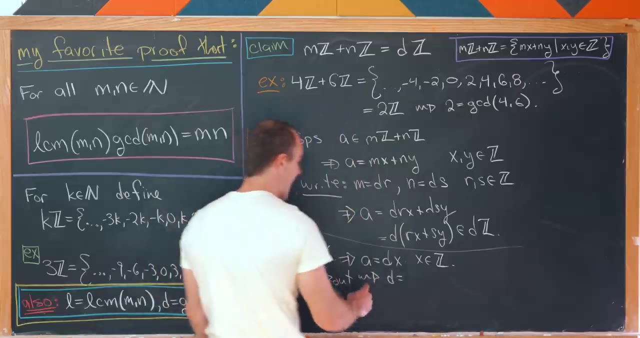 well, I'm going to reuse x, but it is probably a different x than we had up here. So a is equal to d times x. Also, Baizu's lemma, or Baizu's identity, tells us that we can write d as a linear. 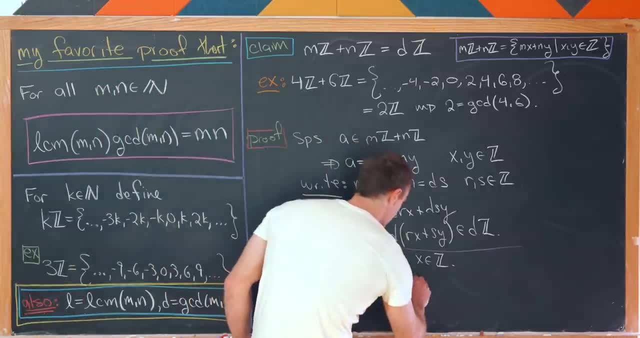 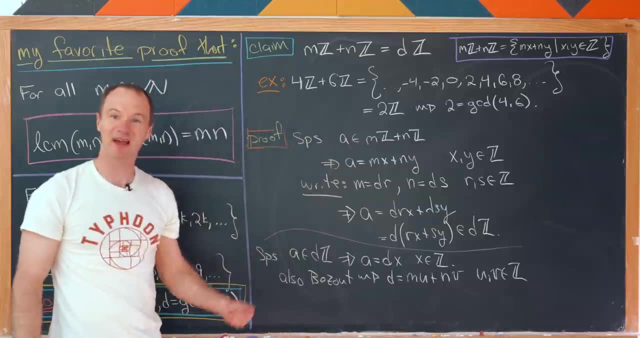 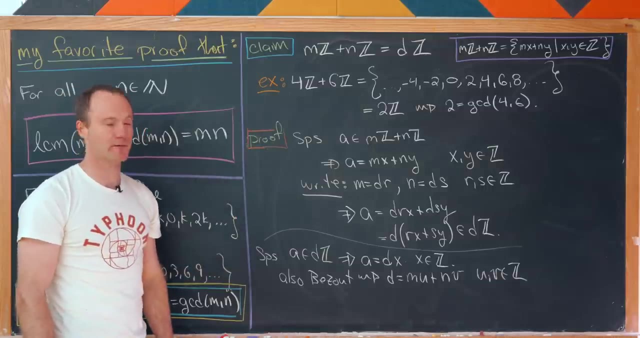 combination of m and n, So maybe we would write it as mu plus nv, as u and v are just some integers that make this happen. Again, that's Baizu's lemma, or Baizu's identity tells us that we can always be written as a linear combination of the two integers. But now we'll interject this. 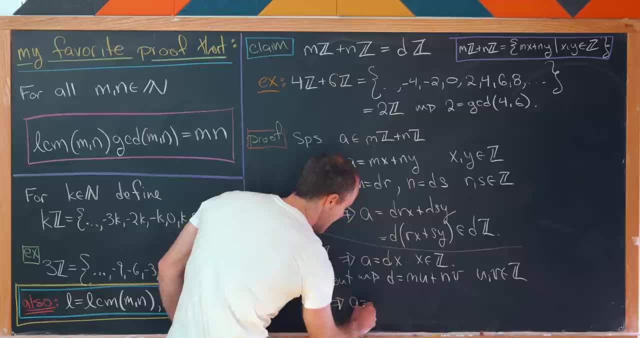 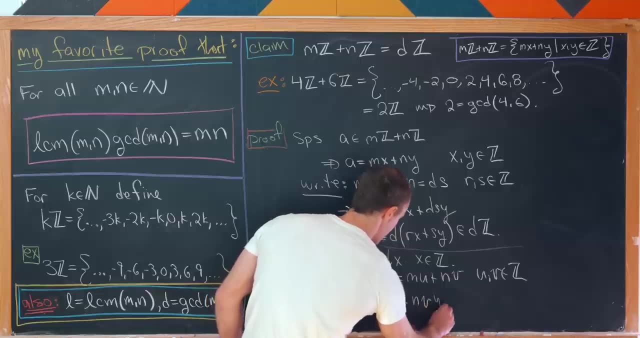 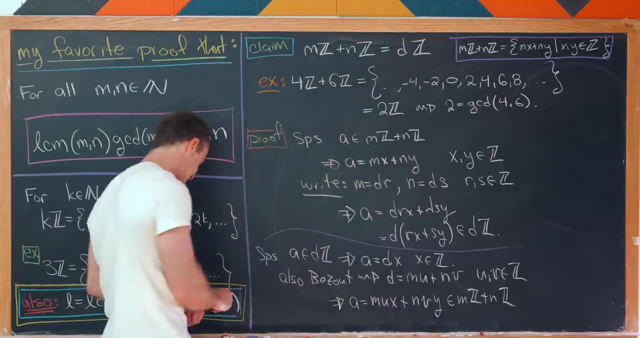 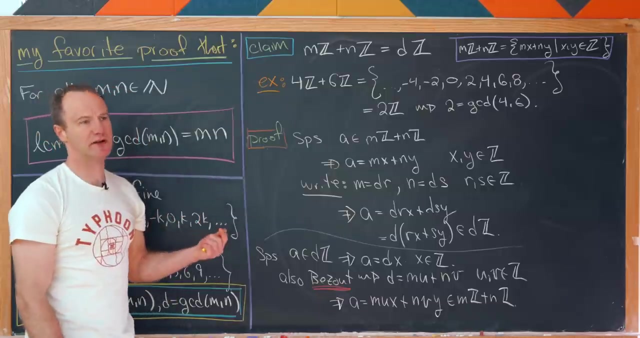 into our equation above and we'll have a is equal to, let's see, m u x plus n v y, But that's most definitely in m z plus n z. So of course we used this identity right here, but it is an identity, or like a result, that we use on the channel a lot when we're solving. 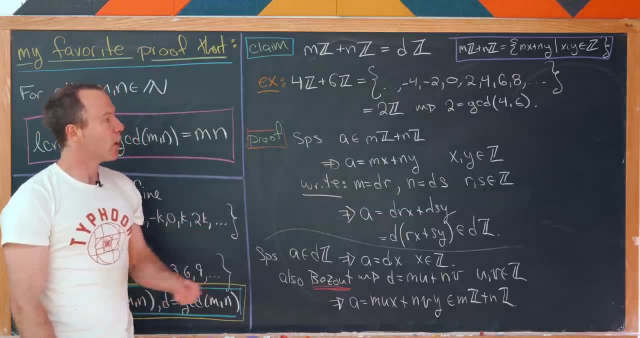 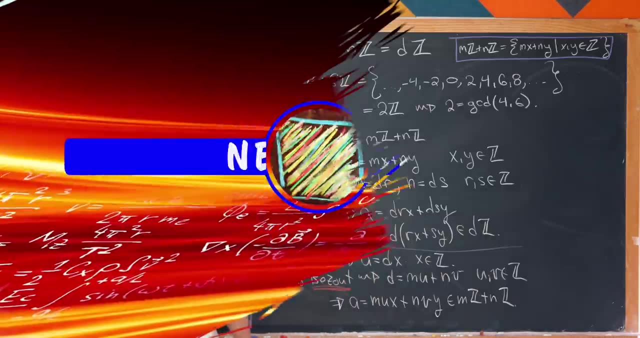 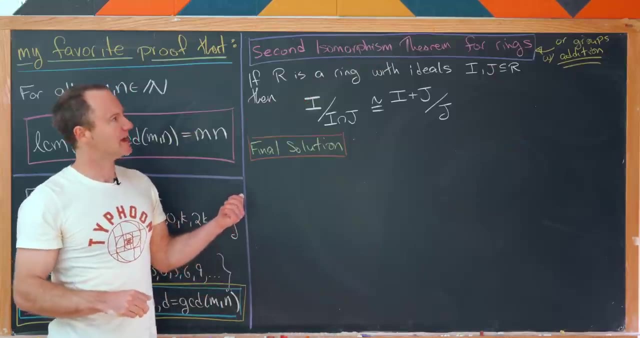 number theory type problems. So I think it's fair. Okay, so now we're ready to look at the proof of our result using a bit of fancy machinery. Now here's where you see that you've been tricked because I've got kind of a fancy theorem on the board. But that being said, 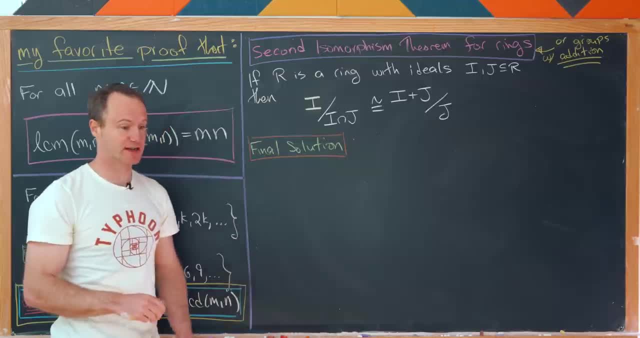 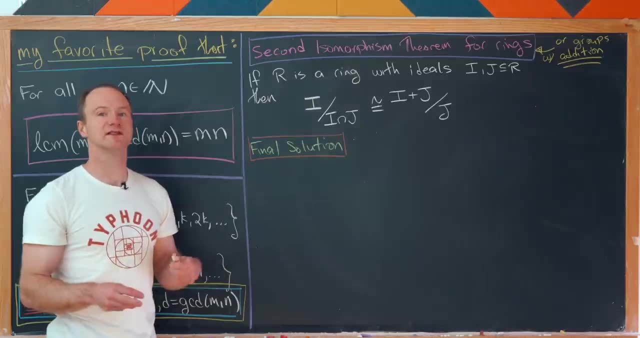 this fancy theorem comes from the coarse abstract algebra And I've got that whole thing in my second channel. And what's the best thing about my second channel? Well, it's got lectures covering full standard courses that you might see in a college or university, And 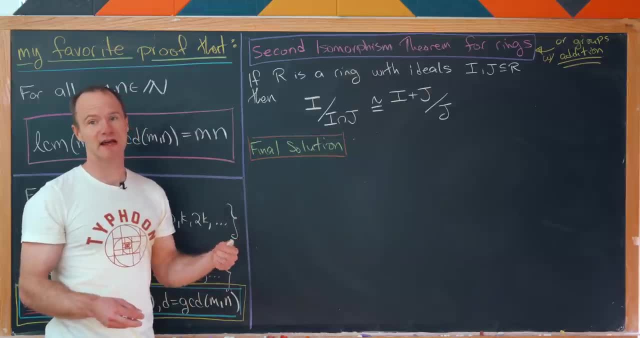 furthermore, there are no ads. And how are there no ads? you might say, Well, it's by our patrons. And if you'd like to help us keep those videos ad-free, thus removing all of the friction to learning mathematics over there on that second channel, consider joining the Patreon. And if 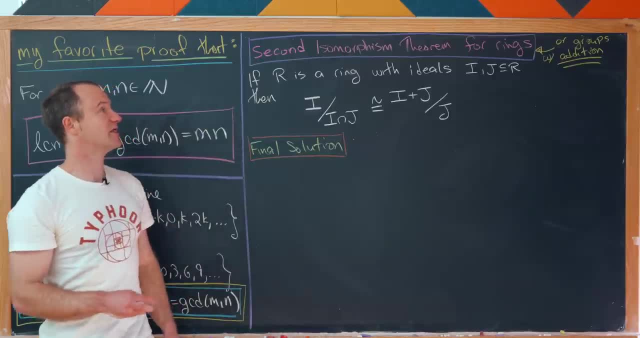 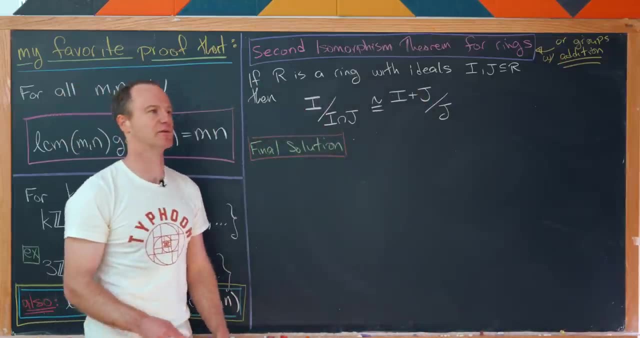 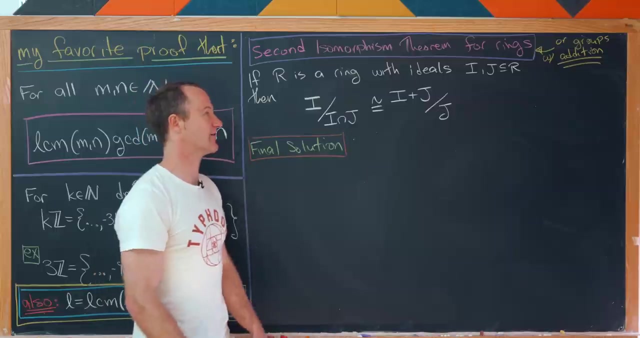 you can't, that's no big deal either, Okay? so anyway, let's look at this, The second isomorphous theorem for rings, Or really, this is also an application of the second isomorphism theorem for groups, applied to additive groups. So let's say we've got a ring R and we have ideals I and. 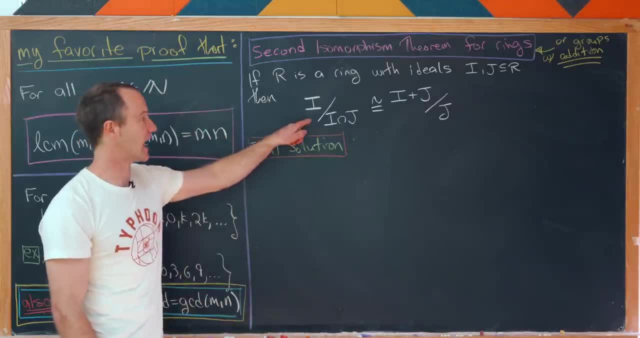 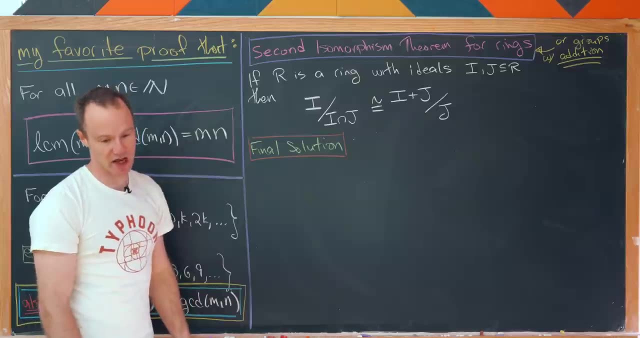 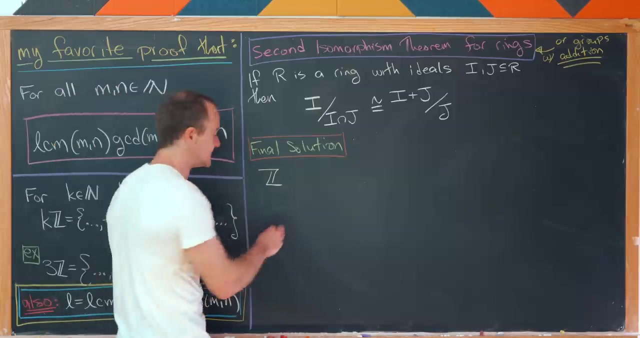 J. Then the quotient ring I mod I intersect J is isomorphic to the quotient ring I plus J mod J. Okay, so now let's just essentially get to it. So we have the ring Z N over D, or you could think of that as an additive group if you wanted to. 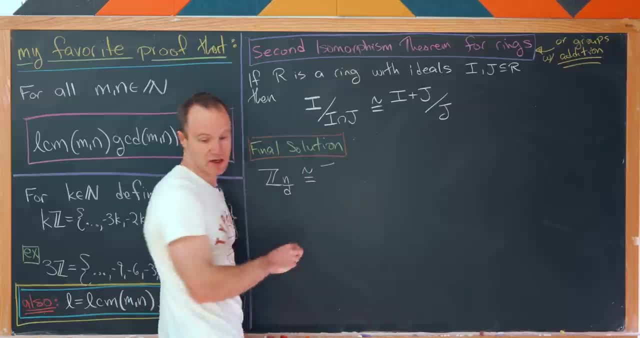 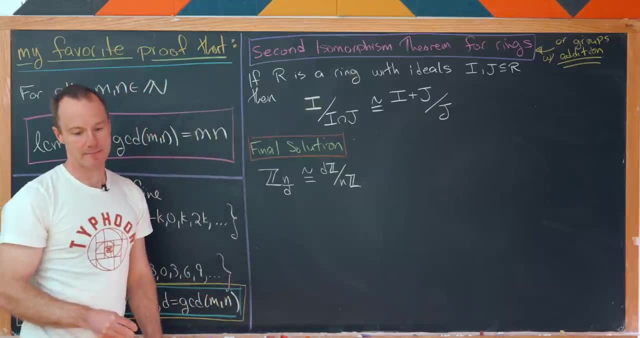 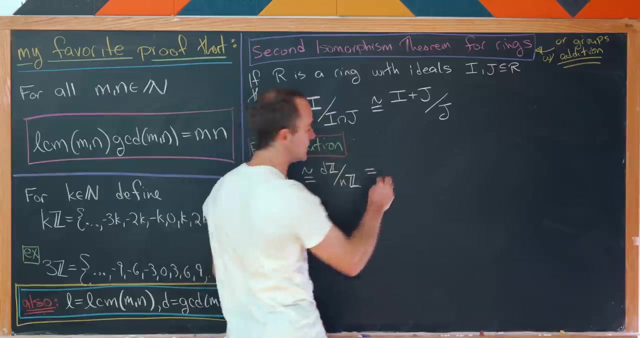 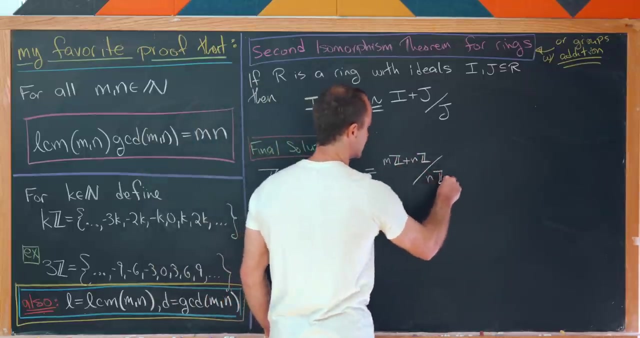 So that's sort of clearly isomorphic to DZ mod NZ. Okay, but then DZ by our result that we had before was equal to MZ plus NZ, And so we have MZ, nz mod nz. This is really good news, because previously we showed that mz. 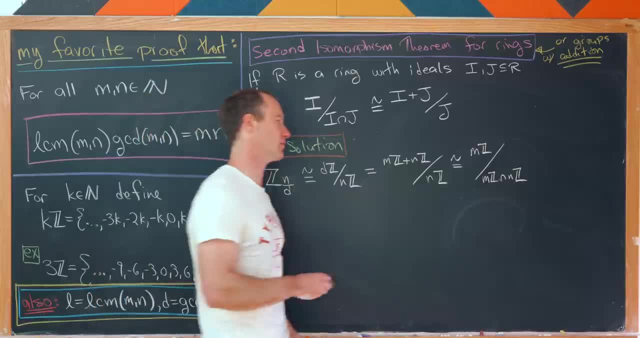 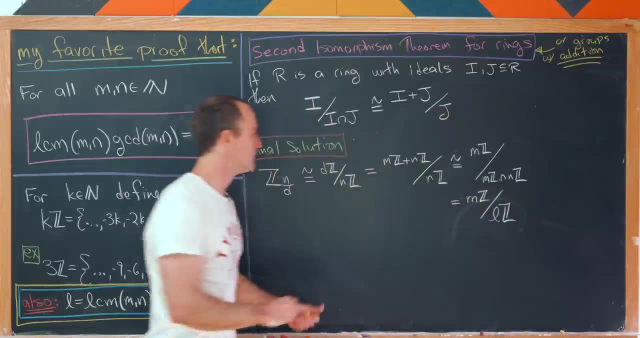 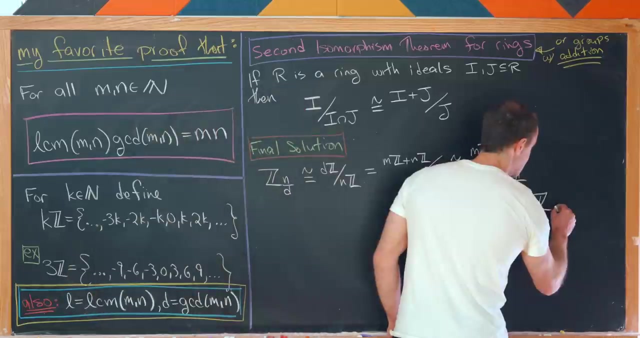 intersect nz was simply lz, where that was the least common multiple. So in fact, here we have: this is just the same thing as nz mod lz, But now, applying this gain in reverse, we see that this is in fact the same thing as z l over m. Okay, 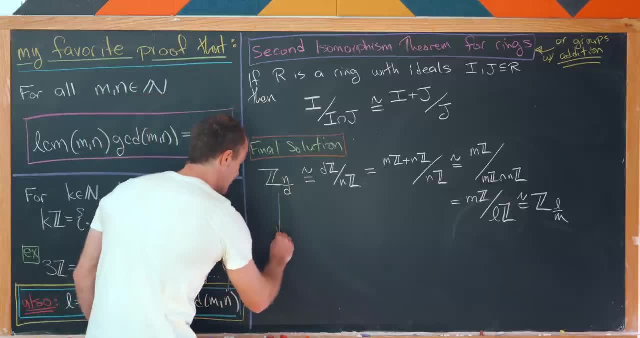 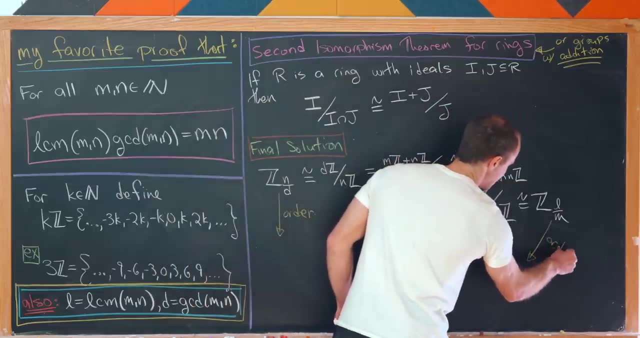 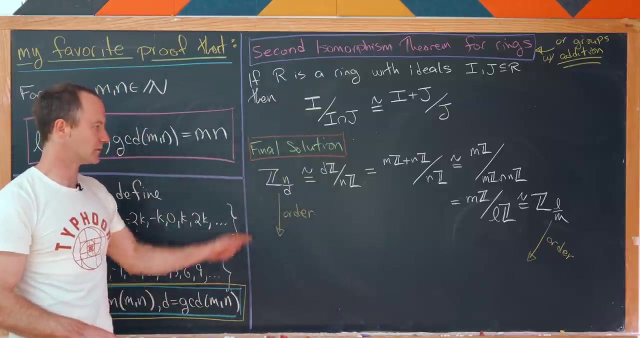 so then, finally, what we do is take the order of these two groups. So we've shown that these two groups- or rings, I should say- well, depending on the setting you're working in- are isomorphic, but if they're isomorphic, they have the same order. So 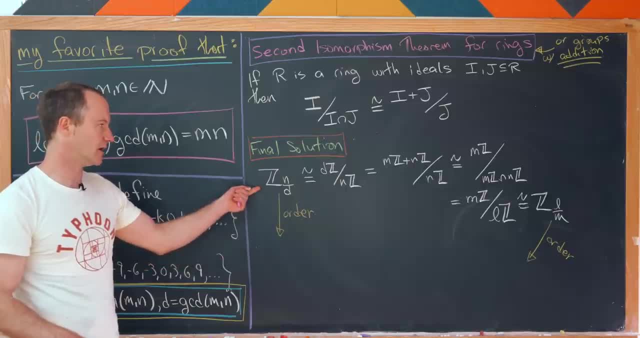 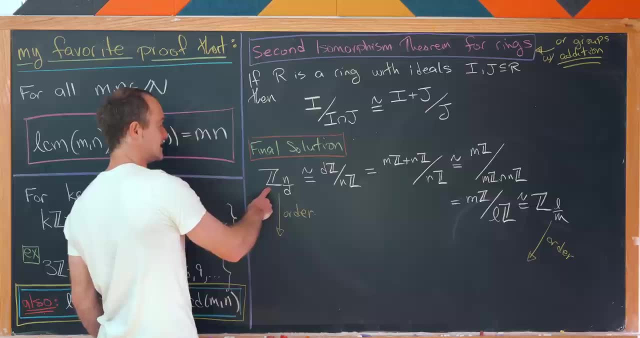 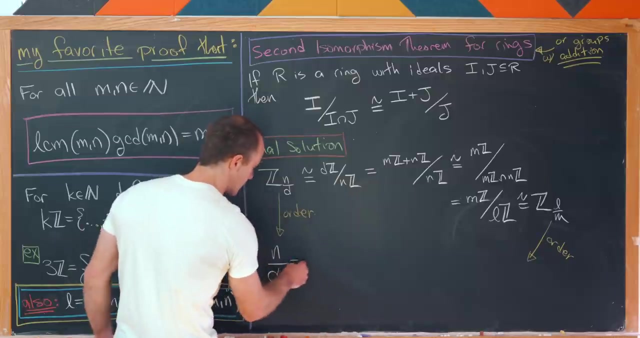 now what we do is just calculate their order. but it's well known that z, you know, blank has whatever that blank is as an order. So in fact, z n over d d has order n over d, whereas z l over m has order l over m, where i've brought this arrow way over. 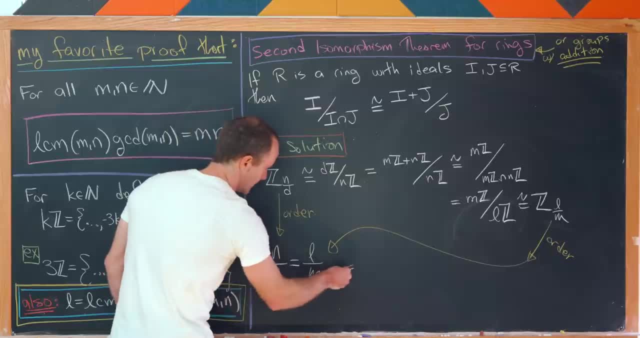 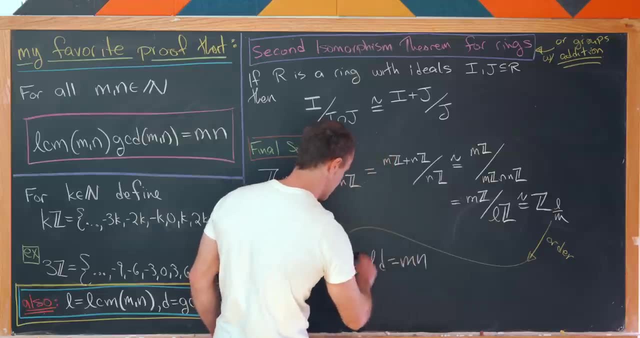 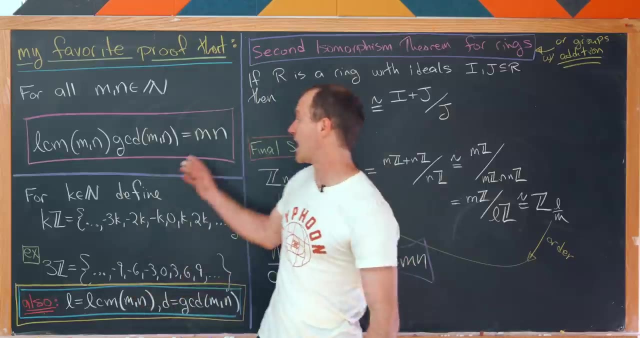 here great. but then we can do a very simple arithmetic problem to get that l times d is equal to m times n. but now check it out using the fact that l was the lcm and d was the gcd. we have achieved this formula over here and that's a good place to stop. thanks for watching and sticking. 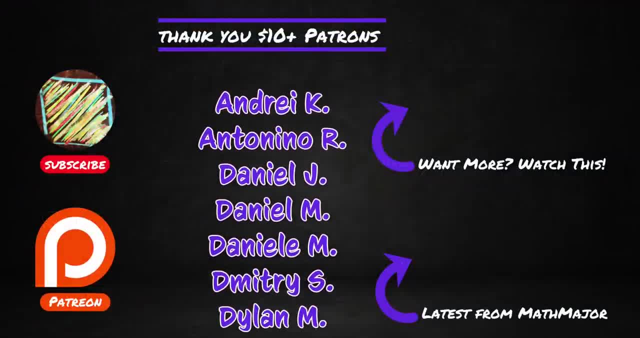 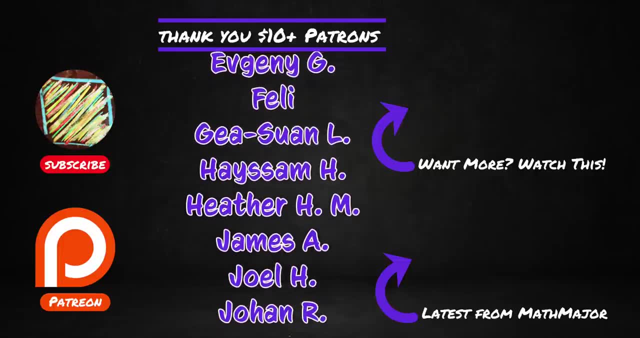 around until the end of the video. and since you're here, don't forget to gently press that like button subscribe, ring the bell and select all notifications to never miss a video, if you want to get your name in the credits, like you see here. access the live seminar series: review videos before release and. 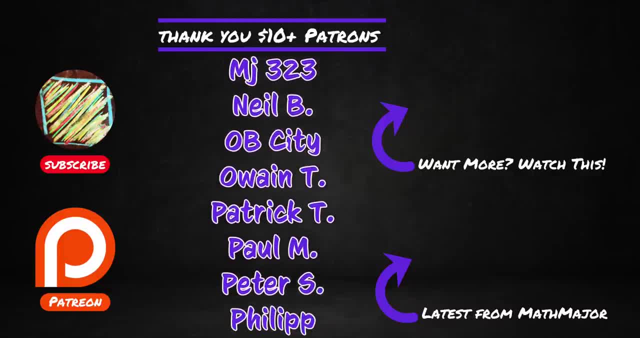 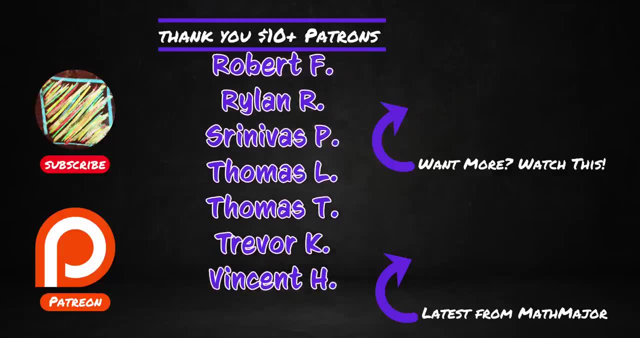 more. go to patreoncom. slash michael pin math and become a patreon member today. if you want full ad free course content, subscribe to my second channel, math major. i've got courses on linear algebra, complex analysis and proofwriting, among several others, and that's everything, bye.